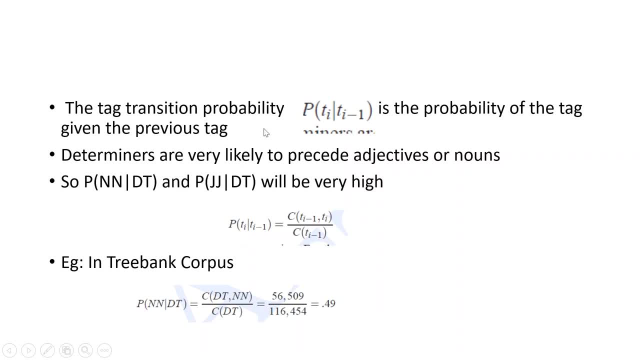 the first is the tag transition probability: Probability of pi given pi minus 1.. It is a probability of the tag given tag, given the probability of the previous tag. So how do we calculate that? Again, all probability calculations are based on some corpus, So we are assuming we have got a data. 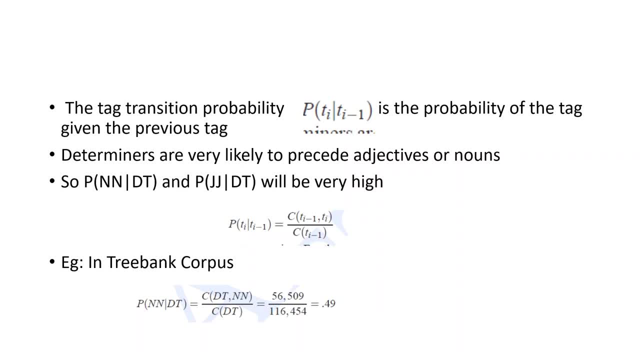 set or a corpus in which we have got lots of words or sentences which you have collected from somewhere. There are standard data sets and we look at. based on that, we look at how the calculation is done. Okay, so in order to calculate this particular value, probability of ti given ti minus. 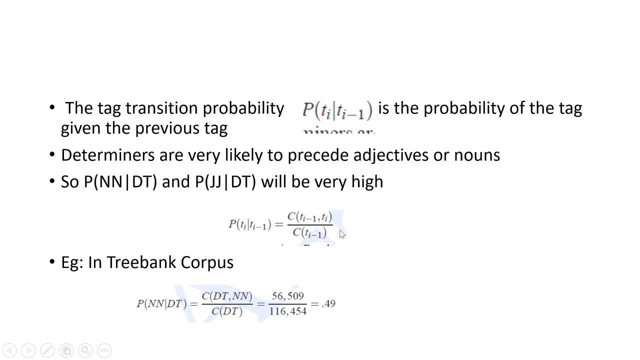 1. What you do is that is, you look at the data set and find out how many times or the count of the number of times the tag ti minus 1 exists in the particular corpus, And then you also find the count of the number of times ti occurs. 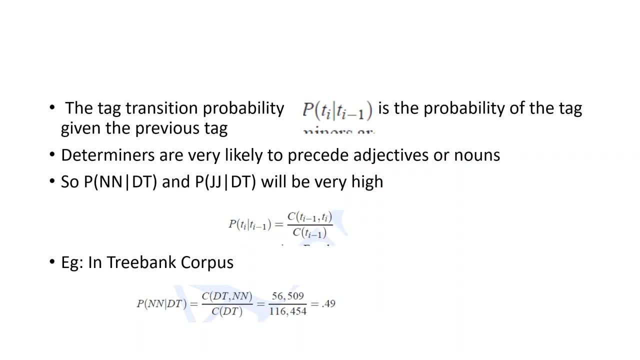 given ti minus 1 occurs just before. Okay, so that is so. basically, you find the counts. Okay, say, for example, in the tree bank corpus, you have got these tags: NN stands for noun and DT stands for determinant. Okay, Now, in order to calculate NN given DT, okay, what is the probability of NN? 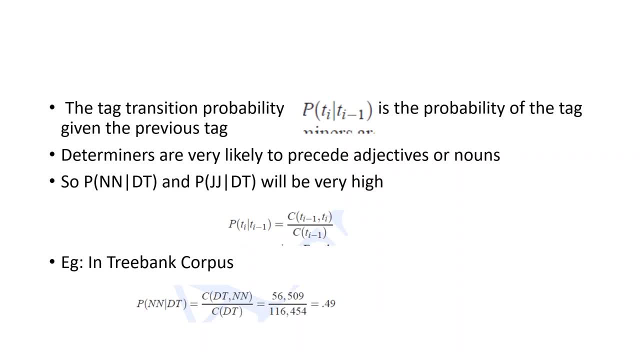 occurring, given that DT occurs before it. So you find out what is the probability of determinants. Okay, What is the count of determinants in the particular tree bank data set? That is, according to the data available, it is 11600454.. Again now, what you look is found from the 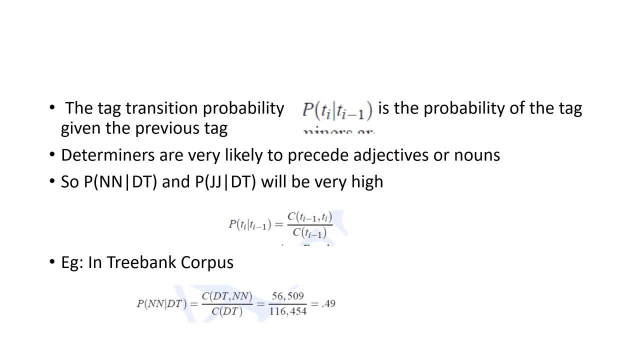 data set itself, find out the count of determinants, given the noun occurs, say after it the cat, Okay, It is after, actually, Okay, The cat. So what is the probability of a determiner given that a noun occurs after it? So that also you find, and finally you have this particular 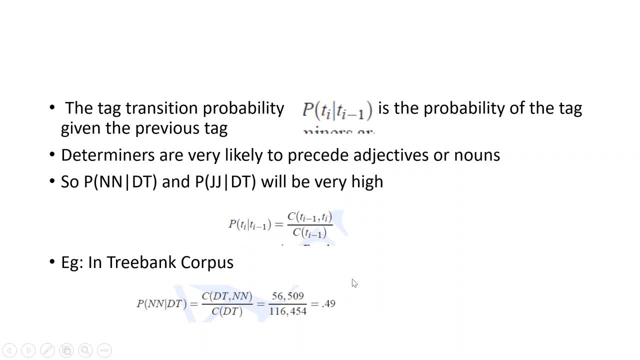 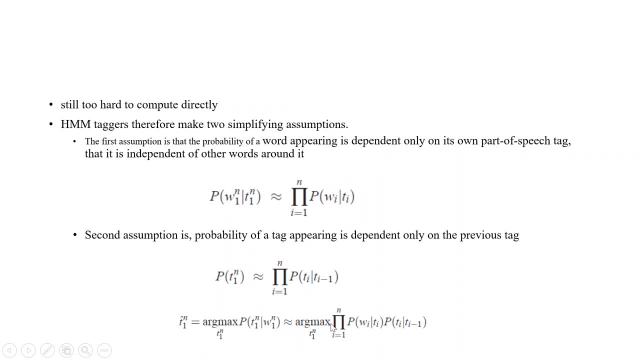 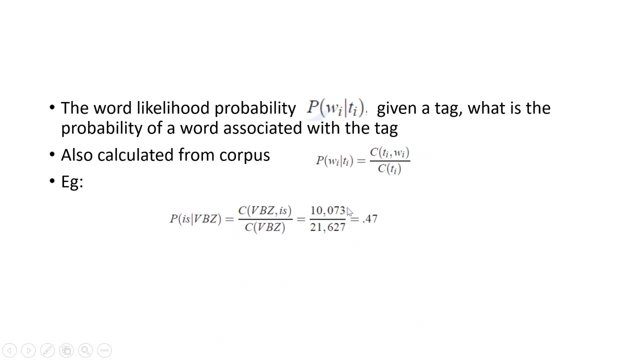 value 0.49.. So determiner occurring before a noun is actually very probable. it is 0.49.. Similarly, the other part of it is probability of a particular word occurring given a particular tag. okay, This also, you actually calculate from the data set. So probability of w i d 1, t i is equal. 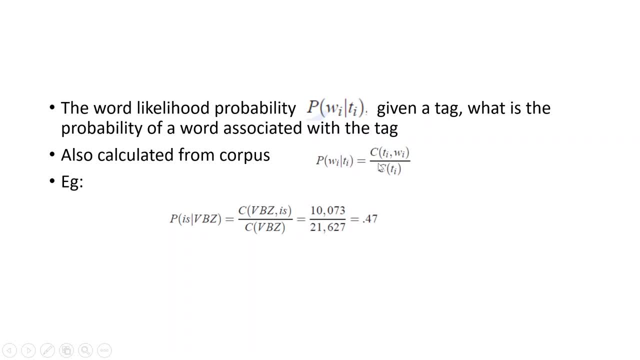 to that is count of t i s in the denominator. How many times does this tag? it is a noun tag in the data set. how many times does the noun tag occur in total, and out of which, how many times does it occur along with this particular word? Say, for example: probability of is given v, b, z. 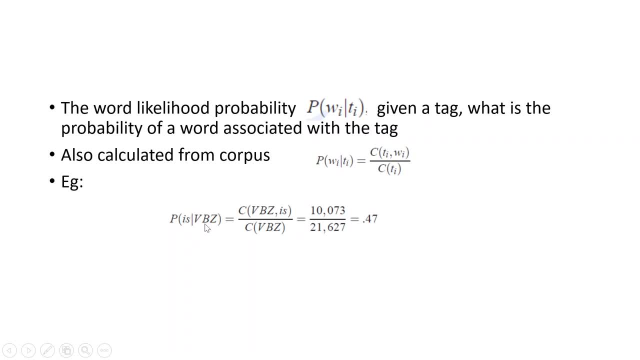 v b z is actually verb third person singular. that is what this tag stands for in the tree bank orders. okay, So probability of is given. v b z is equal to. you find out from the data set how many times, or what is the count of the number of times, the verb in third person singular 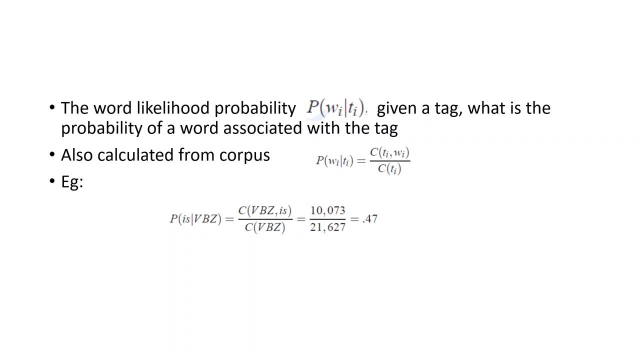 occurs in total in the whole data set. and then, and what is the number of times you have this particular tag for corresponding the word is: So you calculate the count and you find out this. okay, And finally, what do you have? okay, So this is how the probabilities are calculated. 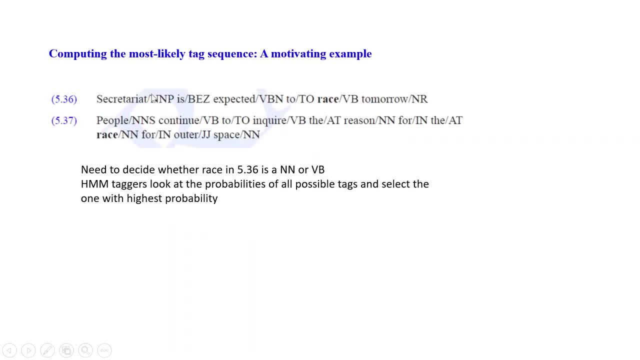 okay. Now, given an example like this: say we have a sentence like this: how do we find out? We said that we. what we do in the probability based tagging is we find out all possible tag sequences and find the probability, the one with the highest probability. How do we? 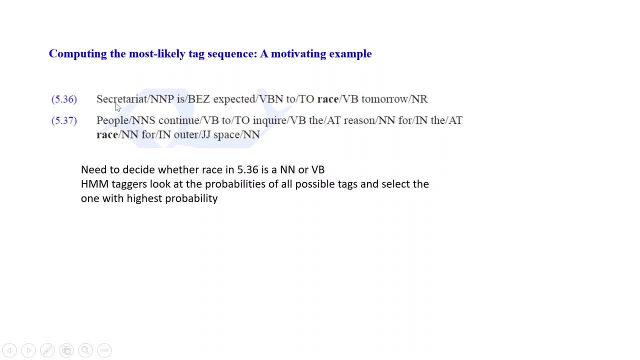 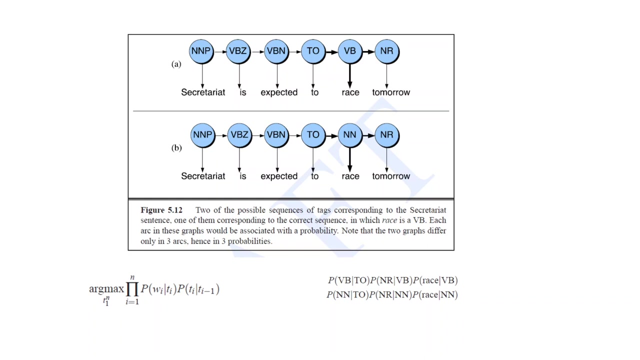 do that, Maybe for this particular sentence: okay, Secretariat is expected to raise tomorrow, okay, And then each word has a corresponding, a probable. the possible tags are available with us and we want to find the one with the highest probability. okay, Now, how do we do that? Okay, Now, if you. 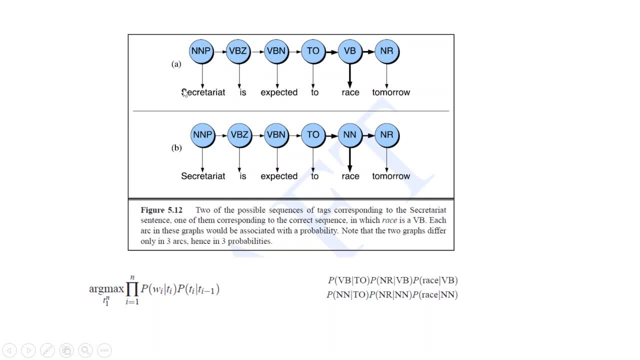 look at this figure. these are two possibilities. These are not the only possibilities. you can have lots of possibilities, but these are two of the possibilities and we try to find out what is the possibility for each of them and see which one is greater. okay, That is what. 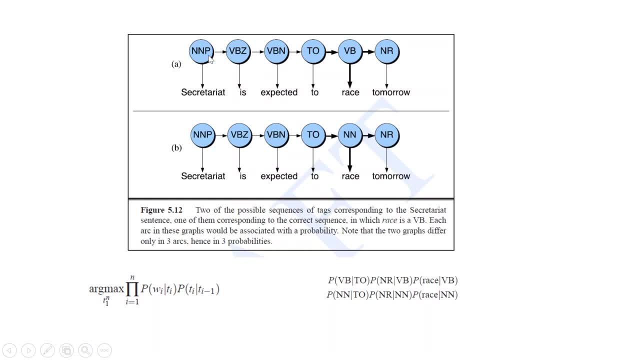 we are going to do okay. So here Secretariat is expected to raise tomorrow. That is our sequence of words and correspondingly, this Secretariat can be now. So if it, if you look at these two examples, the only difference for the tags is only corresponding to this. raise, Raise can be either of these two, or raise can be, say, raise can be higher or raise can be higher. So at a lower tag the only difference is, for example, for the tag it has to be raise can be higher or raise can be higher. Okay, So here you usually see that raise can be high. 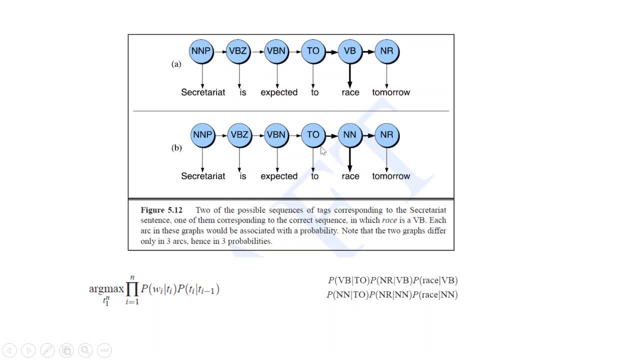 verb or a noun. so in this particular sequence or this particular example, for easiness of understanding we are just changing two of the tags. actually, any of the any of these tags can be vary in any possible combinations, but for ease of understanding we are only looking at. 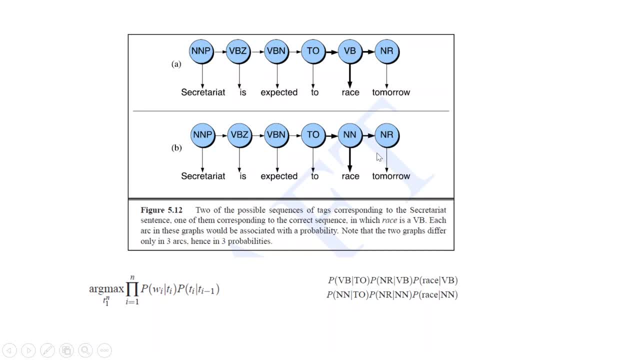 race, having in one sequence it has verb and in another sequence it has noun. now this is our calculation, right, in order to find out the tag with the greater probability. you calculate this. so how do we calculate now, since this is the only place where change happens in the sequence? so, uh, what is given is uh, probability of word wi. given ti into probability. 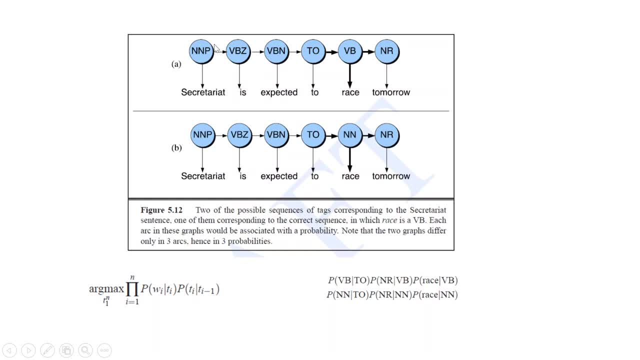 of ti, given ti minus one. you have to find probability of uh, this word, given uh, this word, secretariat, given this, you have to find probability of this word, given this word, secretariat, given this word, this tag, into probability of ti, given ti minus one, and into uh- probability of uh, this word, given. 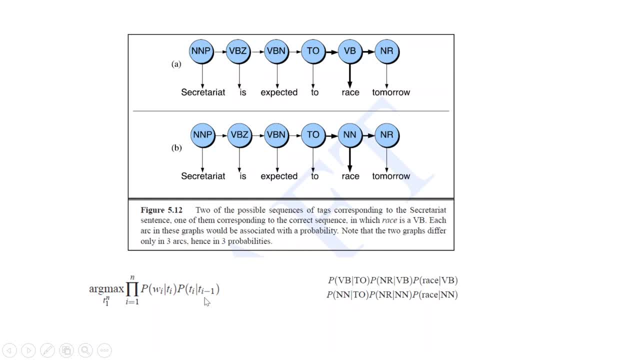 is in the probability of ti given, like that is our sequence and actually. but here we are only looking at this particular point. there is a difference in there. okay, our difference is only in the difference. so only that we are looking at. if it is greater than that, we take it as a tag sequence. 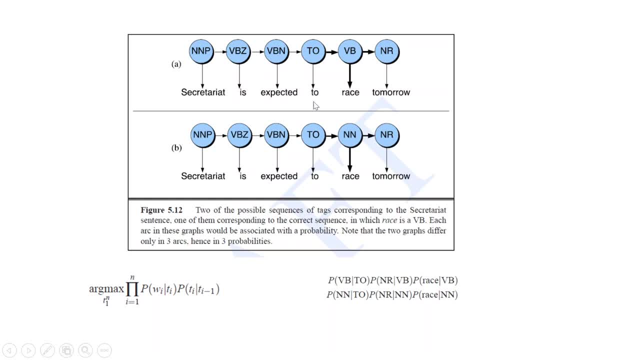 that is the idea here. okay, so the only change that happens is in this transition probability: t, i, t, t, i, minus one tag in the transition problem team. here the transition probability will be different. okay, similarly, uh, this transition and this transition is different. and also here, all the.